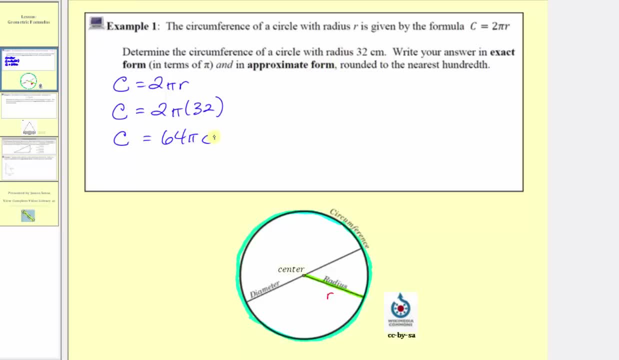 and because the radius is in centimeters, the circumference is also in centimeters. So this is the exact circumference. And now to approximate the circumference, we'll actually do this two ways. A common approximation for pi is 3.14, but most calculators also have a pi key. 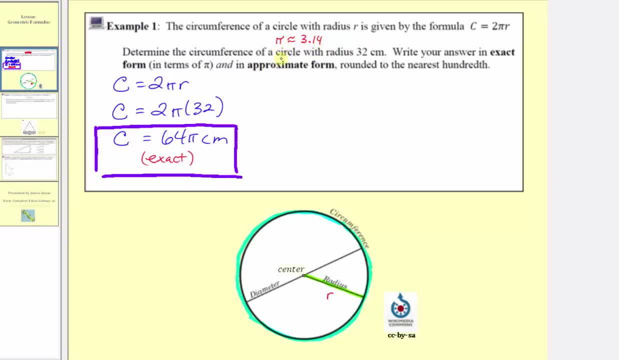 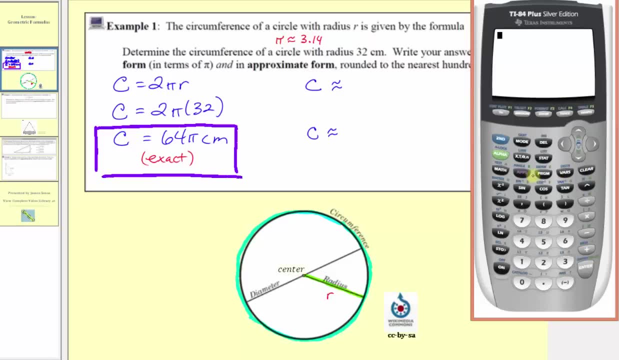 which would give a more accurate approximation for pi. So we'll determine the approximate circumference using both methods. So, going to the calculator, let's first use the pi key on the calculator, which would give us a more accurate approximation, So we'll enter 64, and then to access the pi key, 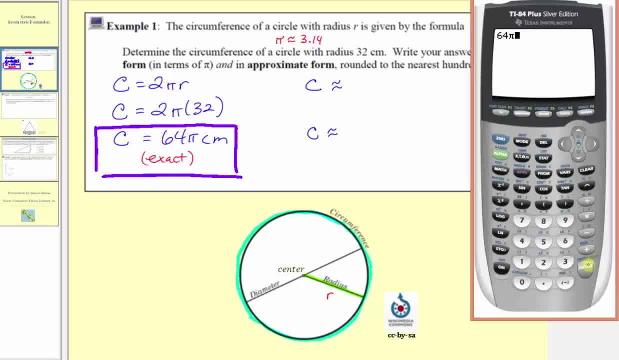 we press second and then the exponent key here, and then the exponent key here, and then the exponent key here, and then enter To the hundredths place value, because we have a one in the thousandths place value. we would round down. 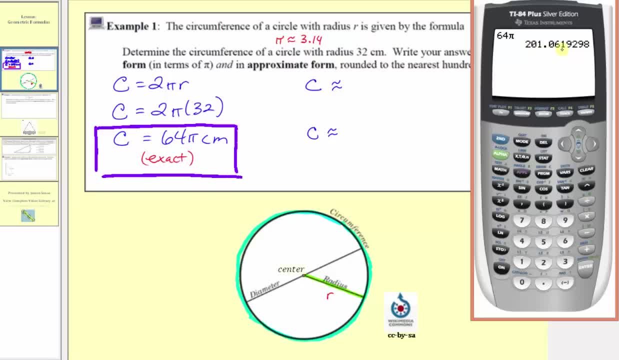 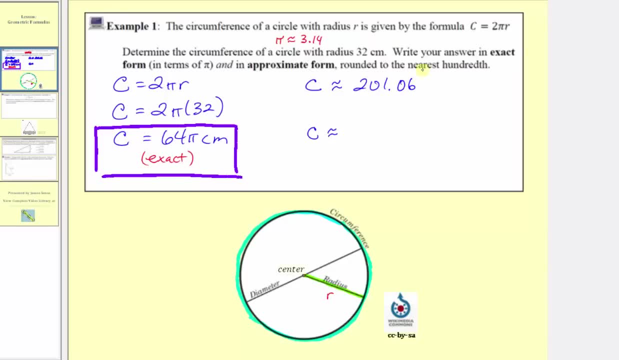 we'd approximate the circumference to be 201.06, or 102 and six hundredths. Let's go ahead and record this Again. this would be centimeters, and this is the approximation using pi on the calculator. Now let's make another approximation. 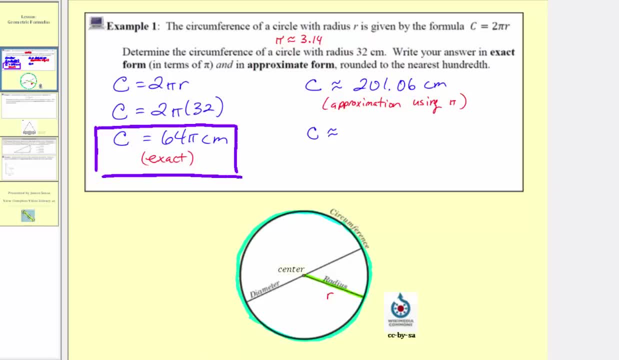 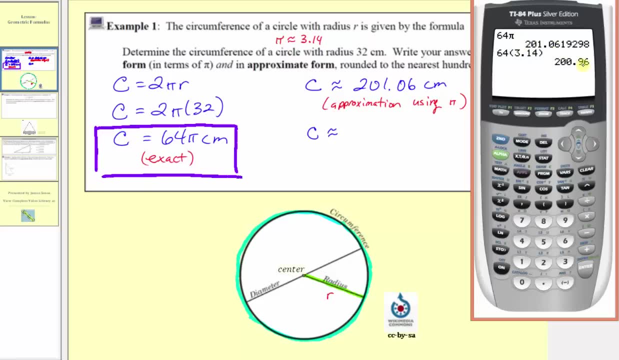 using pi as approximately 3.14.. So we'll enter 64 times 3.14.. So we'll enter 64 times 3.14.. So we'll enter 64 times 3.14.. Notice how it does give us a different value. 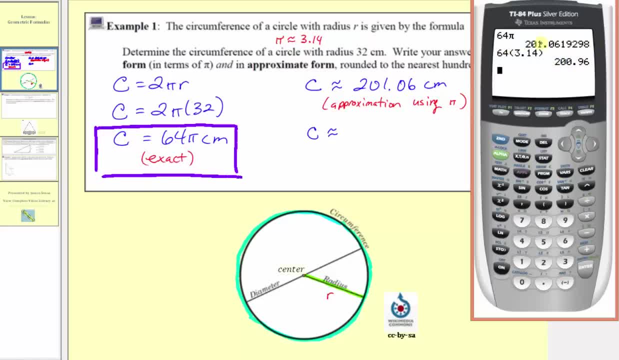 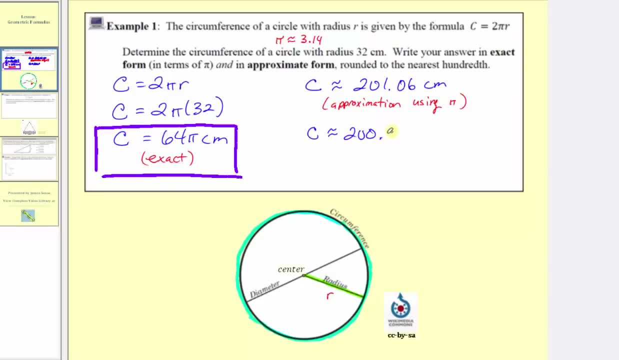 This approximation is not as accurate as this approximation here. So our second approximation is going to be 200.96, or 296 hundredths centimeters, And we'll say: this is the approximation, using pi as approximately 3.14.. using pi as approximately 3.14.. 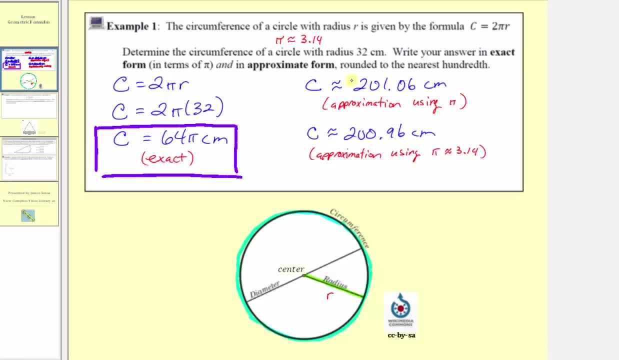 So it is important, when doing the whole thing or doing your homework, to read the directions carefully. My suggestion would be to use the pi key on the calculator, unless it indicates to use a different approximation for pi. In example two we're told the formula. 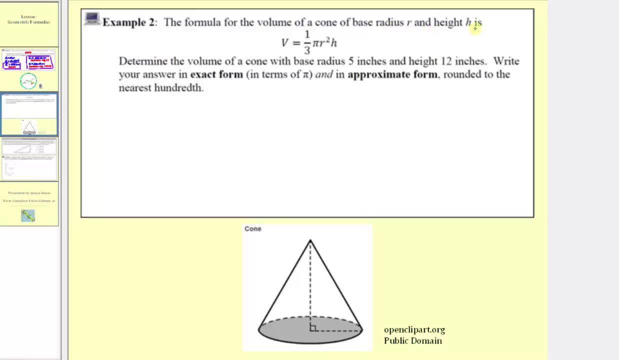 for the volume of a cone of base radius r and height h is given by v equals one-third pi r squared h. A cone is pictured below. This length here would be the height and this length here would be the base radius. We're asked to determine the volume of a cone. 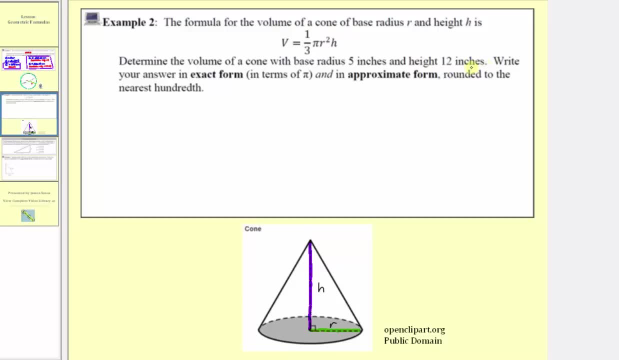 with a base radius of five inches and a height of 12 inches. So because we're determining volume, we measure volume in cubic units, so our volume is going to be in cubic inches. We're asked to write the exact form in terms of pi. 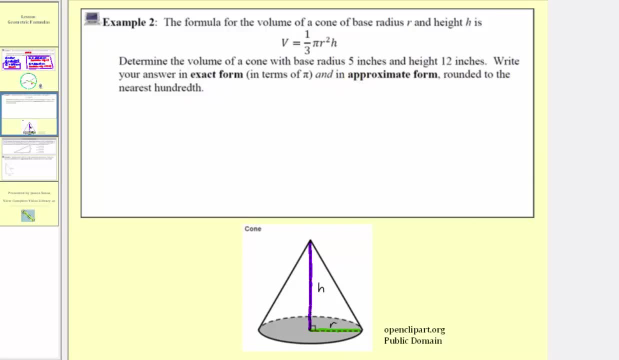 and also an approximate form to the nearest hundredth. So, beginning with the volume formula, the volume v equals one-third pi r squared h. We'll substitute five for r and we'll write: v equals one-third pi r squared h. So the volume is equal to one-third pi times five, squared times 12.. 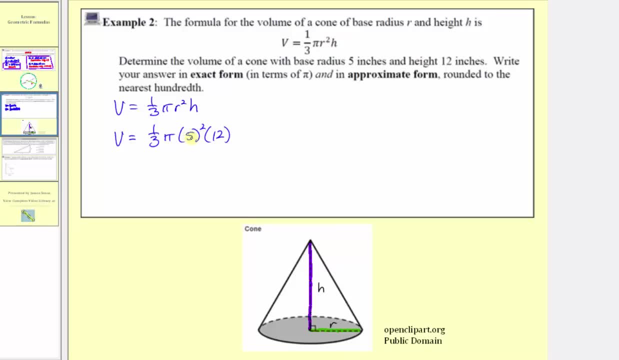 Now, following the order of operations, we would simplify the exponents. first. Five squared is equal to five times five or 25.. So we'd have the volume: v equals one-third pi times 25 times 12.. Now before we multiply though, 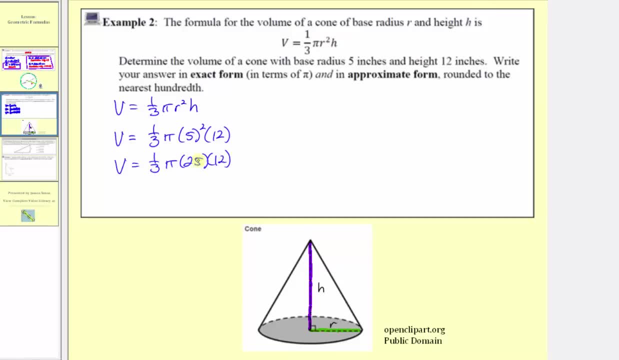 because we have a fraction here. notice how, if we write 25 times 12 as a fraction with a denominator of one, we should recognize we are going to have a common factor of three between three and 12.. There's one three in three and four threes in 12.. 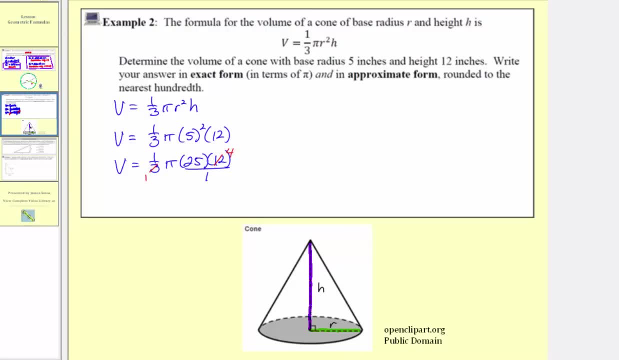 And now we can multiply. Notice how the denominator is one which means the product is going to be pi times 25 times four, which equals 100 pi. So the exact volume is equal to 100 pi and again the units would be cubic inches. 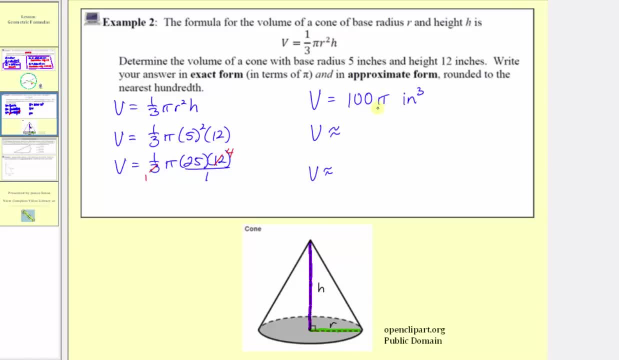 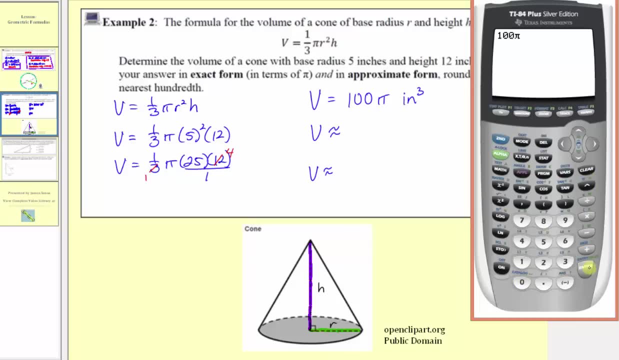 Now let's make our approximations for the volume. Let's first use the pi key on the calculator, So we'll enter 100, and then, using the pi key, press second and then the exponent key enter. Notice, here we have a nine in the thousandths place value. 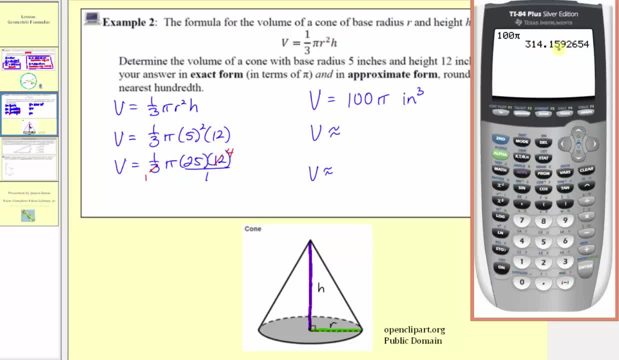 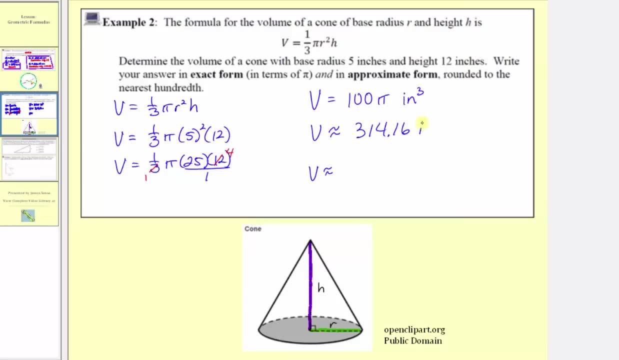 so we round up to 314.16, or 314 and 16 hundredths. Again, this is cubic inches, And this is the approximation using pi on the calculator. And now let's make another approximation using 3.14.. And this one we shouldn't need the calculator. 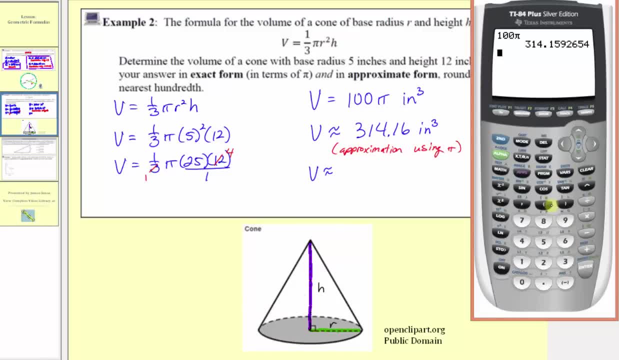 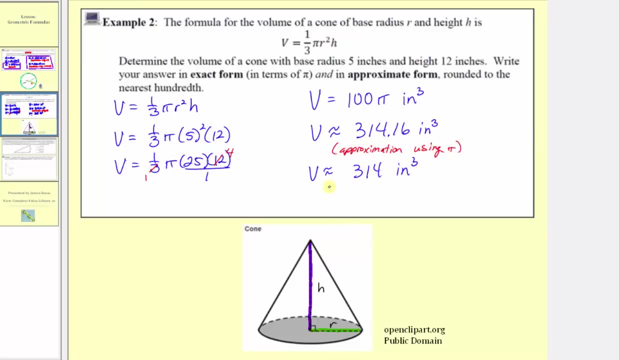 3.14 times 100, we should recognize will be 314.. Let's go ahead and show it: 100 times 3.14 is 314.. Again, this is the approximation using pi. So this is approximately 3.14.. 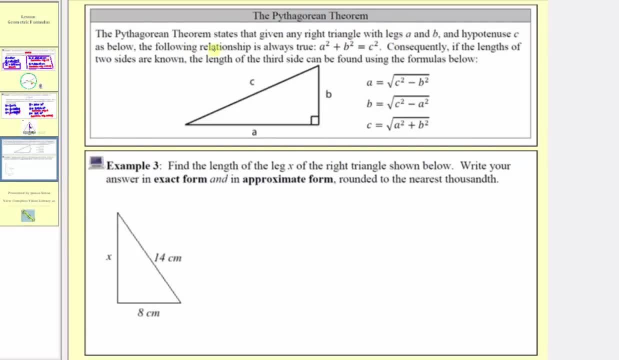 Before we look at example three, let's look at the Pythagorean Theorem. The Pythagorean Theorem states that given any right triangle with legs A and B in hypotenuse C as below, notice how the two legs form the right angle. 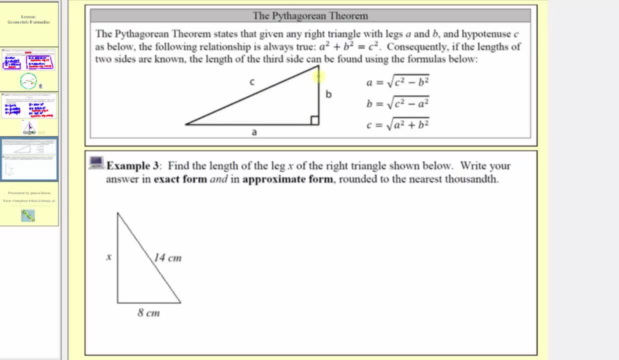 The hypotenuse is opposite the right angle. It's also the longest side of the triangle. The following relationship is always true: A squared plus B squared equals C squared, And we can use this theorem to find the length of one side if the length of the two other sides is known. 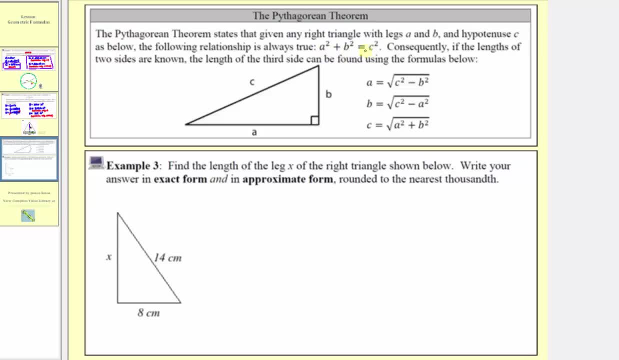 These three equations here are derived from A squared plus B squared equals C squared. We're solving for A, B and C. We're asked to find the length of the leg X of the right triangle shown below and then write the answer in exact form. 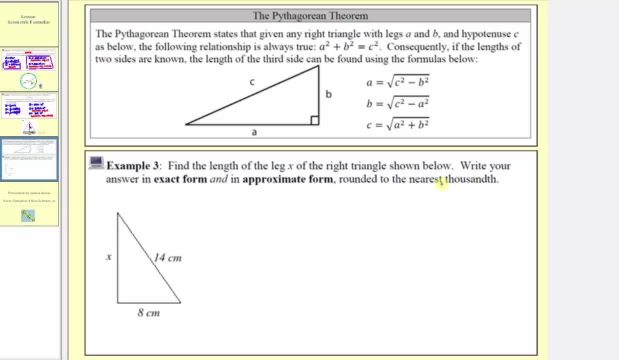 and, in approximate form, run it to the nearest thousandth. Let's first make sure we label the three sides correctly. Remember A and B must be the two legs, So let's let this leg be A and this leg be B. 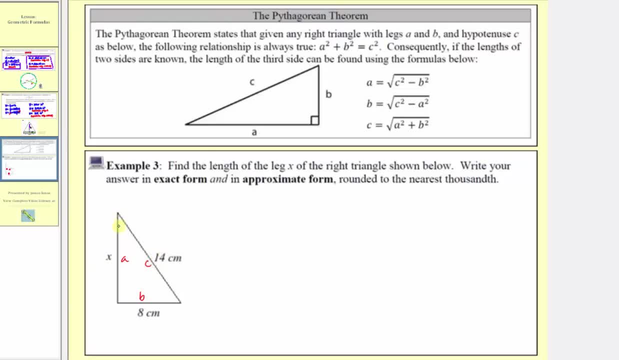 and the hypotenuse must be C, Because we're determining the length of this leg here, which we labeled A. we'll go ahead and use this equation here. that's already solved for A. So we have: A equals the square root of C squared, minus B squared. 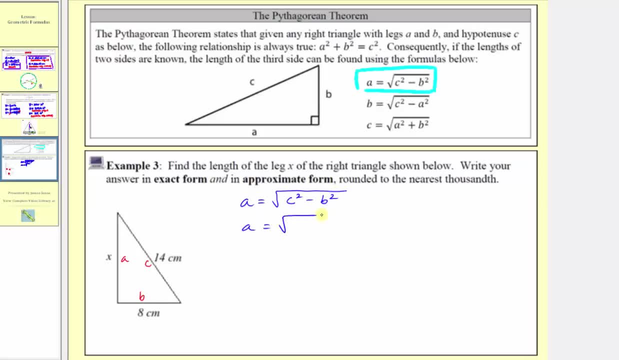 So in our case, we'll have A equals the square root. Well, C squared would be 14, so we'll have 14 squared Minus B squared, which would be eight squared. Simplifying, we have A equals the square root. 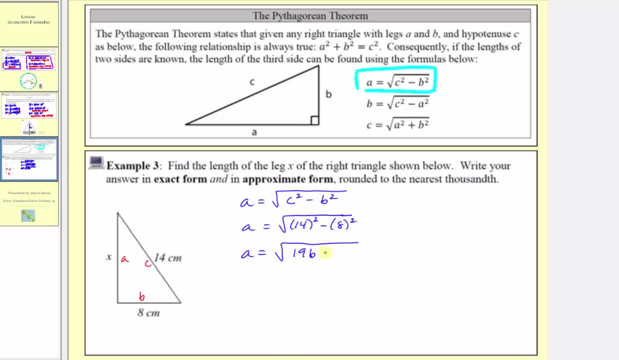 of 14 squared is equal to 196, minus eight squared is equal to 64. So we have: A equals the square root of 196 minus 64 is equal to 132.. So the exact value of A is the square root of 132,. 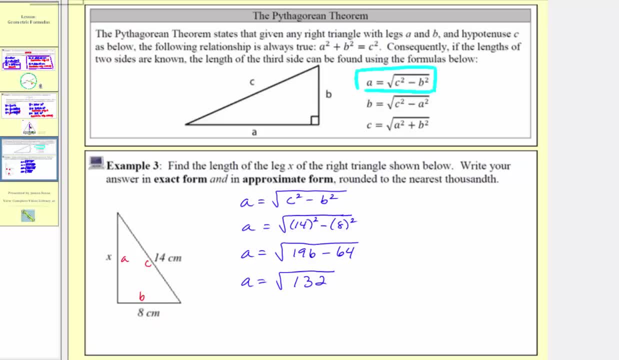 and because the lengths are measured in centimeters, the length of side A is exactly the square root of 132 centimeters, Depending on what classroom you may be able to stop here, but I also want to show how the square root of 132 can be simplified. 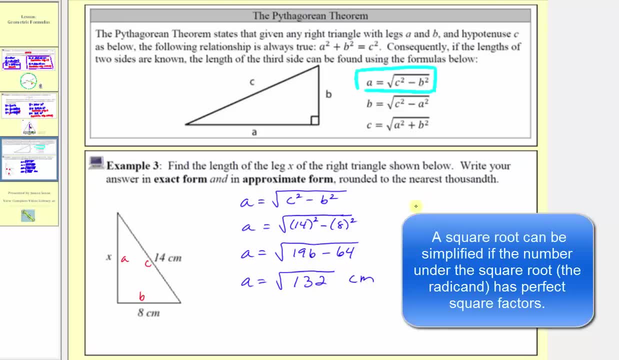 If we look at the prime factorization of 132,, 132 is equal to two times 66,. two is prime. 66 is equal to two times 33,. two is prime. 33 is equal to three times 11, both are prime. 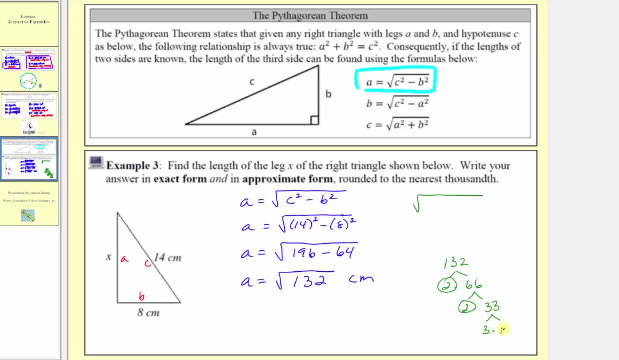 So the square root of 132 is equal to the square root of two times two times three times 11.. But two times two, which equals four, is a perfect square, And we know this because we have two equal factors here. We can simplify the square root of 132 to two times two. 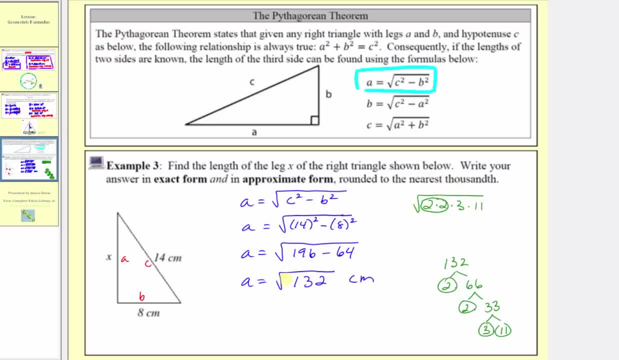 which is equal to two times three times 11.. So we can simplify the square root of 132, to two square root 33.. The two outside the square root came from the square root of two times two, or the square root of four, which equals two. 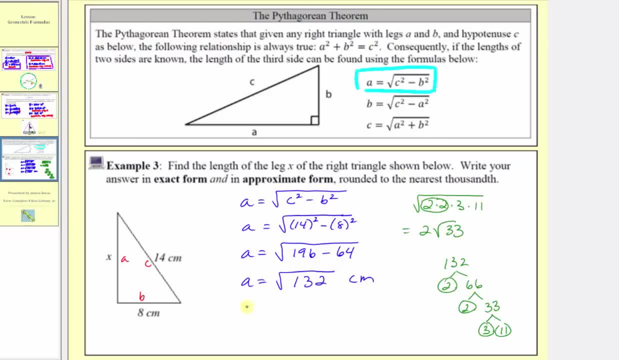 So let's also express the exact length as A equals two times the square root of 33 centimeters. So here are two ways to express the exact length. And now let's also show the approximate form. So we'll go back to the calculator. 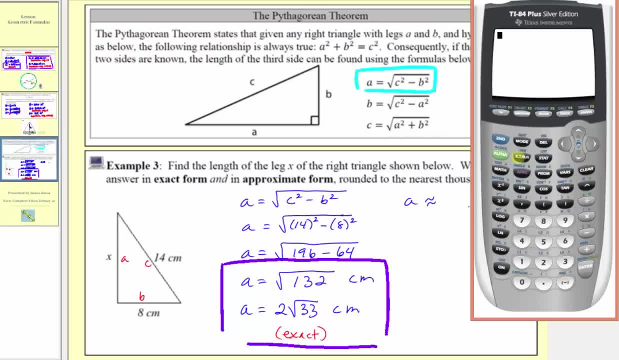 and we can enter either of these two forms. Let's check to make sure they're the same. So second x squared brings up the square root and then we enter 132, enter. Let's also make sure that two square root: 33.